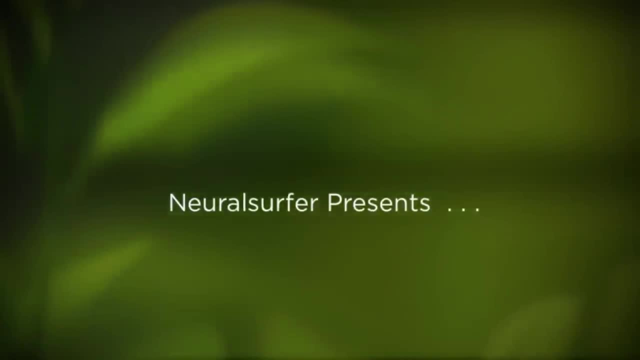 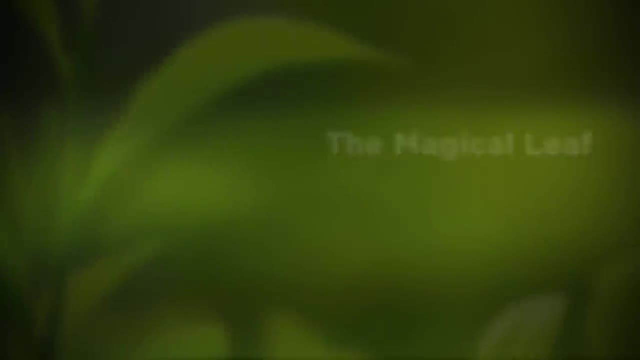 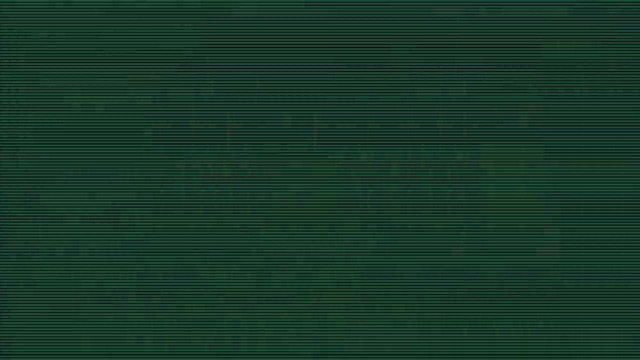 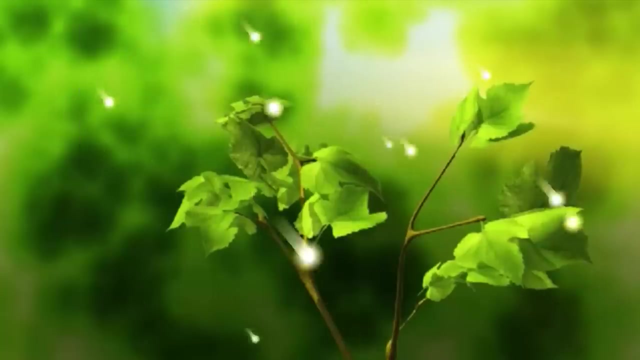 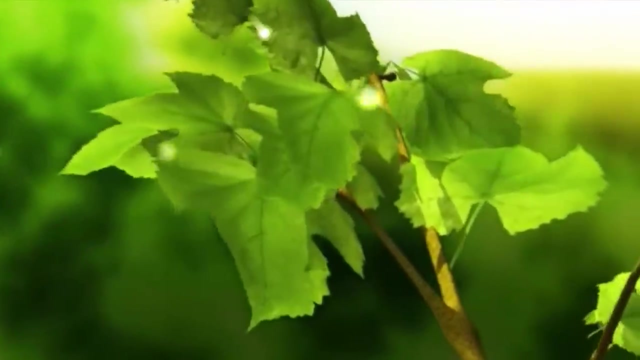 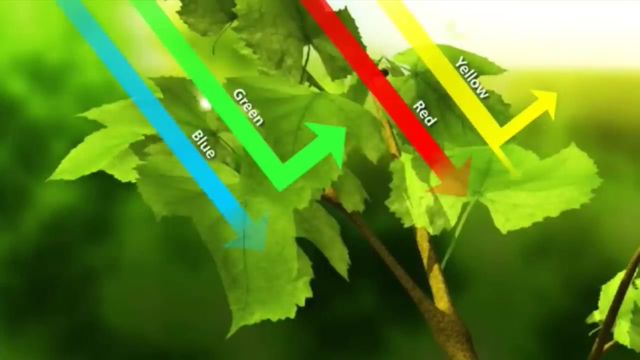 The leaf it turns out is a remarkable piece of technology. Light lands on a leaf in quantum energy packets called photons. Every second it spends in bright sunlight brings a leaf, thousands of trillions of photons And almost every one of the red ones. it's captured and its energy processed. 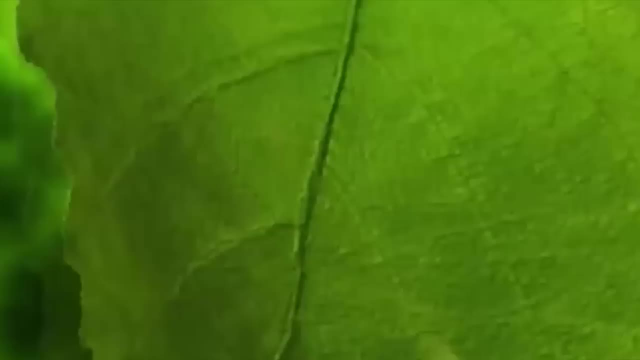 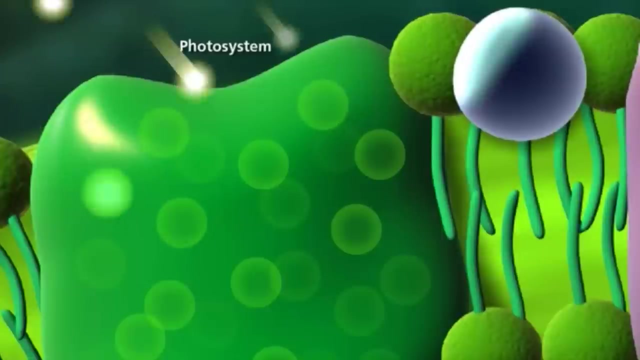 Let's trace the path of that energy through the plant. The first stop is the antenna, an assembly of hundreds of thousands of chlorophyll molecules Hit by the photon. an electron within the chlorophyll will become excited and use the extra energy to bounce through the antenna. 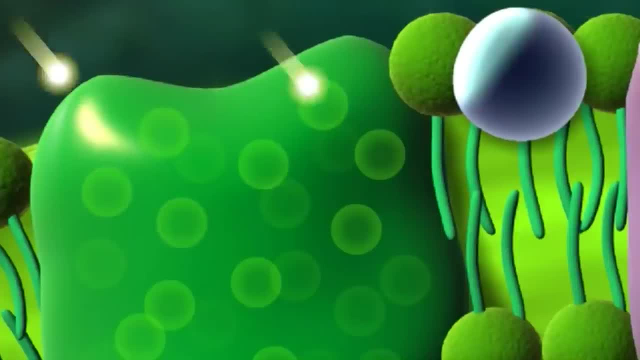 to a bridging area. This is composed of a complicated arrangement of chlorophyll molecules. You can imagine it as an intertwined maze of roped bridges that, if you can find the path through, lead to the all-important reaction center. Once at the reaction center, the electron creates a permanently separated charge. 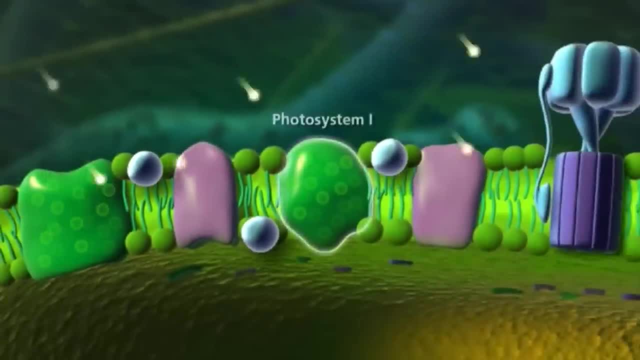 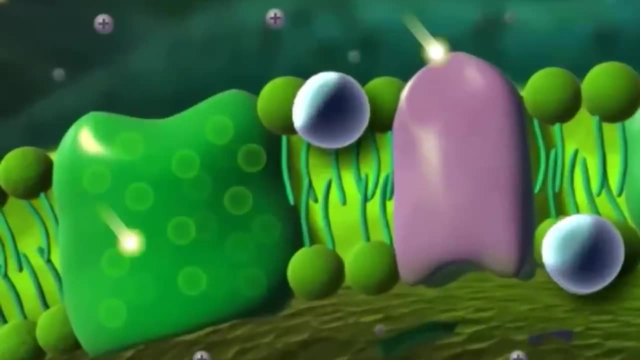 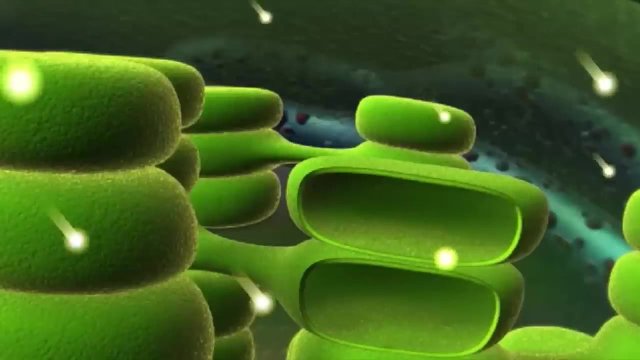 that is essentially energy that can be stored. It's the same thing that makes a fully charged battery such a useful source. At that point, the energy is safe and properly stored, ready for use by the plant. There's just one catch: The reaction center is a nearly impossible place to reach. 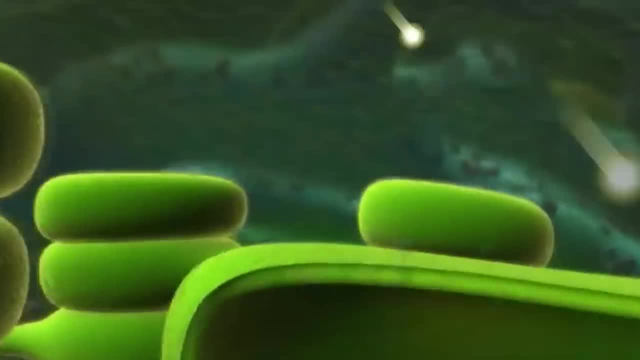 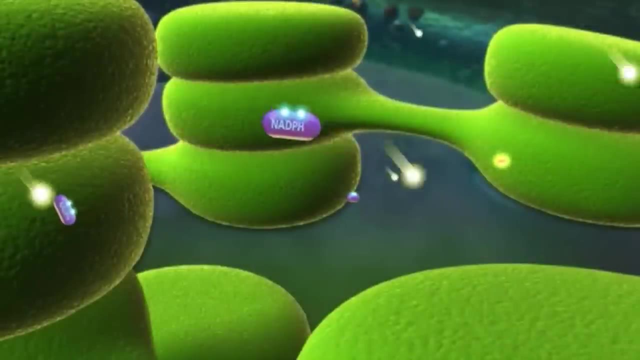 Getting through the bridging area is a nightmare and it has to be done quickly. The maze of wobbly roped bridges will absorb all the photon's energy if it takes too long to find the reaction center. A packet of energy has about one nanosecond to get to the reaction center. 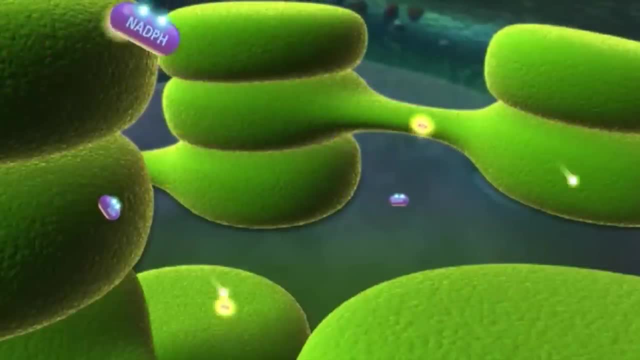 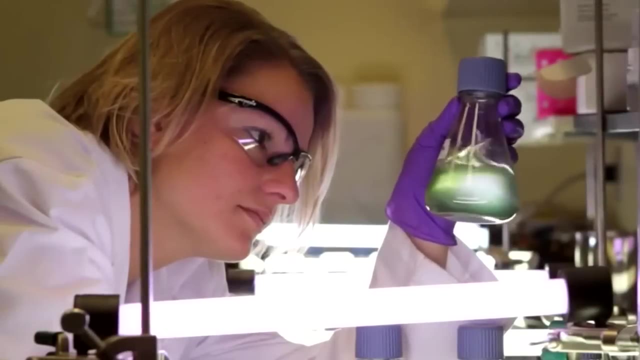 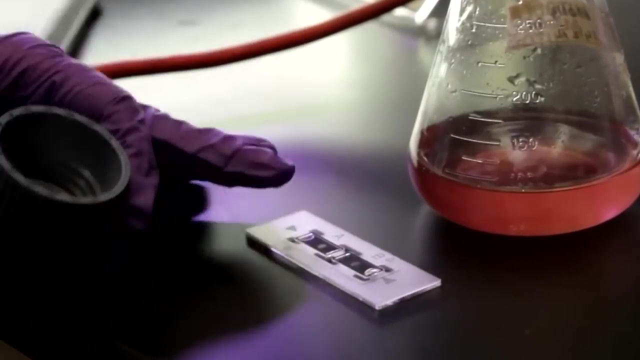 It takes about an hour to find the reaction center. Some might chance upon the right path and make it through in time. Most, though, won't. This is where the quantum tricks and Gregory Scholl's research team comes in Their conclusion.